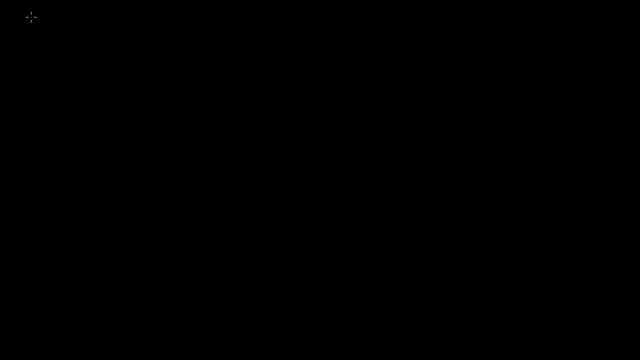 Let's say I've got me a set of vectors, So let me call my set B And let's say I have the vectors v1,, v2, all the way through vk. And let's say: this isn't just any set of vectors. 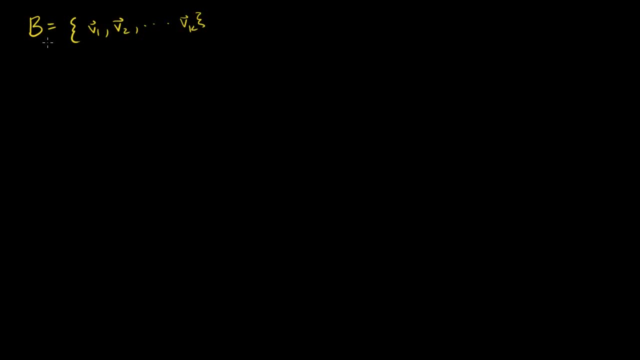 There's some interesting things about these vectors. The first thing is that all of these guys have length of 1.. So we could say the length of vector vi is equal to 1, for i is equal to well. we could say between 1 and k, or i is. 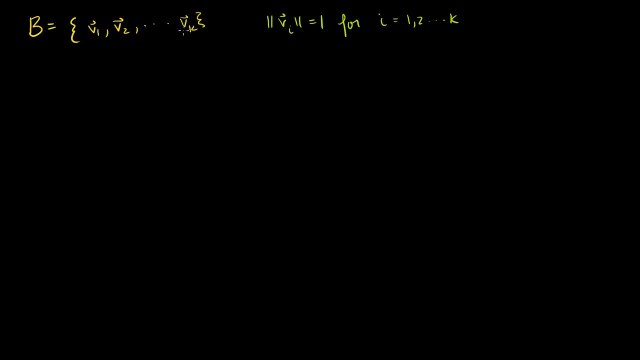 equal to 1,, 2,, all the way to k. All of these guys have length equal 1.. Or another way to say it is that the square of their lengths are 1.. The square of vi's length is equal to 1.. 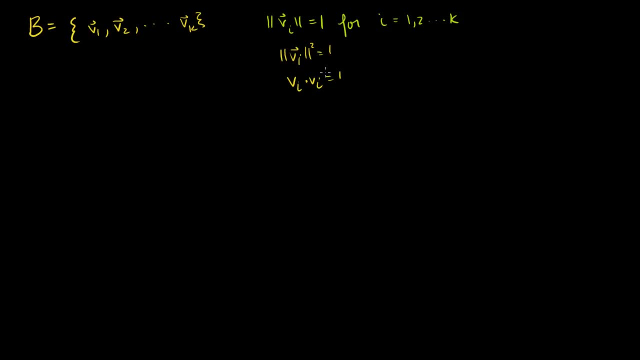 Or vi dot vi is equal to 1.. For i, is you know any of these guys? Any, i can be- 1,, 2,, 3, all the way to k. 4i is equal to 1, 2, all the way to k. 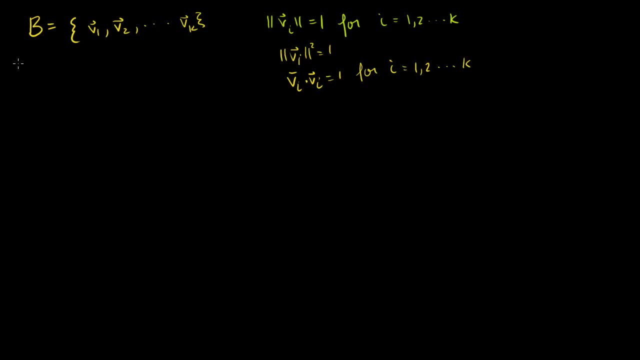 So that's the first interesting thing about it. Let me write in regular words: All the vectors in B have length 1.. Or another way to say it is that they've all been normalized. That's another way to say that Is that they have all been normalized. 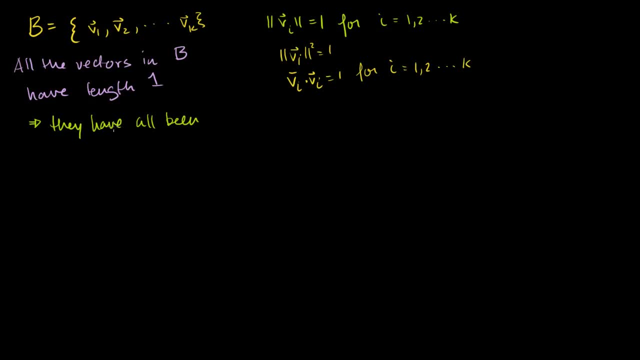 Or they're all unit vectors. Normalized vectors are vectors that you've made their lengths 1. You've turned them into unit vectors. They have all been normalized. So that's the first interesting thing about my set B. And then the next interesting thing about my set B is that 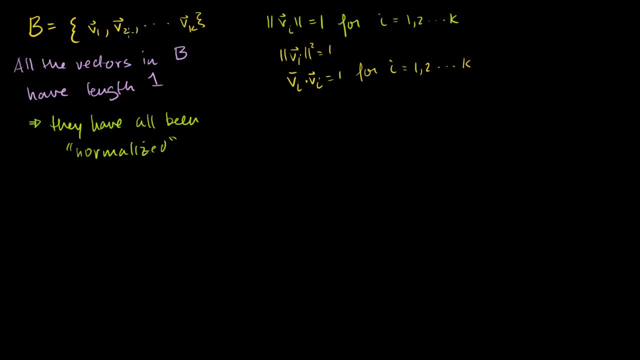 all of the vectors are orthogonal to each other. So if you dot it with itself, So if you dot a vector with itself, you get length 1.. But if you take a vector and you dot it with any other vector, if you take vi and you were to dot it with vj, 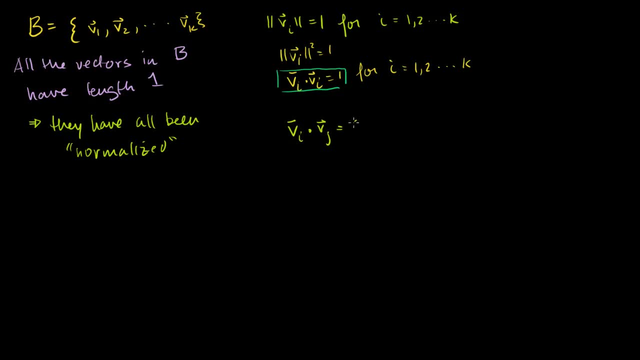 So if you took v2 and dotted it with v1, it's going to be equal to 0.. For i does not equal j, It's going to be 0.. All of these guys are orthogonal. Let me write that down. 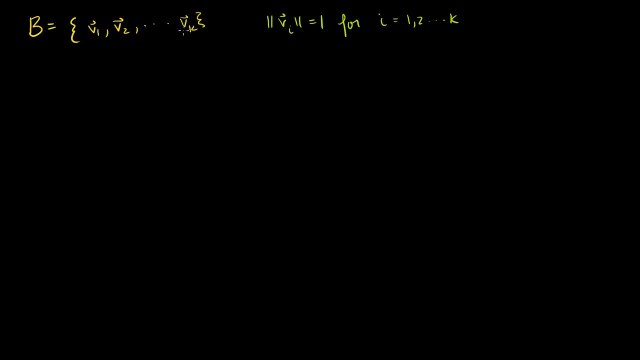 equal to 1,, 2,, all the way to k. All of these guys have length equal 1.. Or another way to say it is that the square of their lengths are 1.. The square of vi's length is equal to 1.. 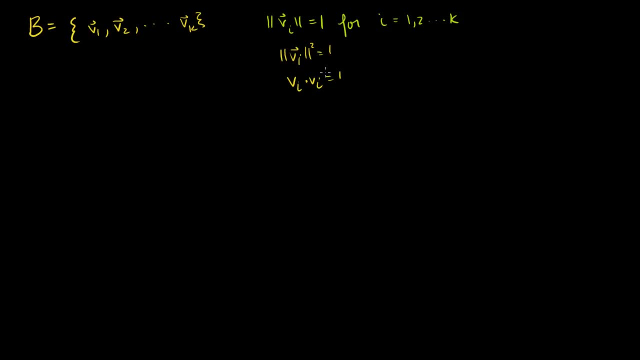 Or vi dot vi is equal to 1.. For i, is you know any of these guys? Any, i can be- 1,, 2,, 3, all the way to k. 4i is equal to 1, 2, all the way to k. 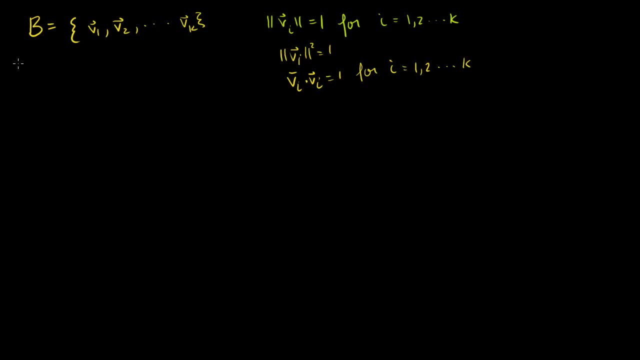 So that's the first interesting thing about it. Let me write in regular words: All the vectors in B have length 1.. Or another way to say it is that they've all been normalized. That's another way to say that Is that they have all been normalized. 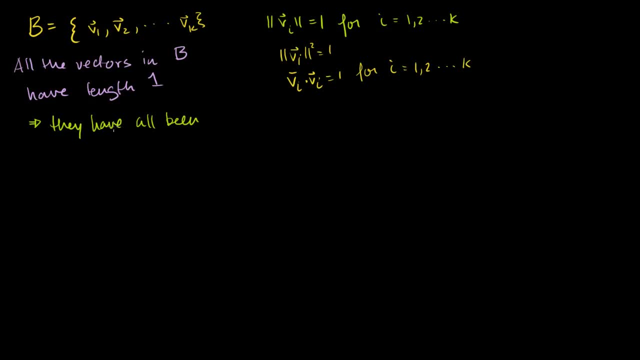 Or they're all unit vectors. Normalized vectors are vectors that you've made their lengths 1. You've turned them into unit vectors. They have all been normalized. So that's the first interesting thing about my set B. And then the next interesting thing about my set B is that 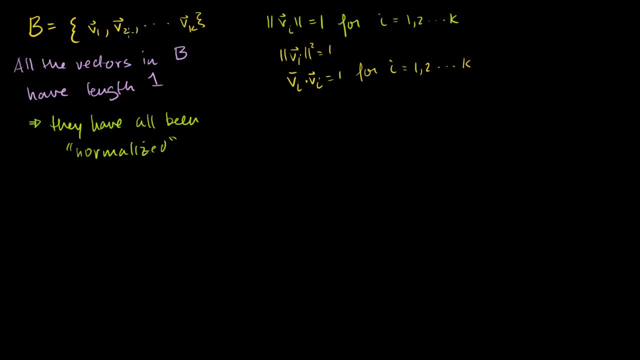 all of the vectors are orthogonal to each other. So if you dot it with itself, So if you dot a vector with itself, you get length 1.. But if you take a vector and you dot it with any other vector, if you take vi and you were to dot it with vj, 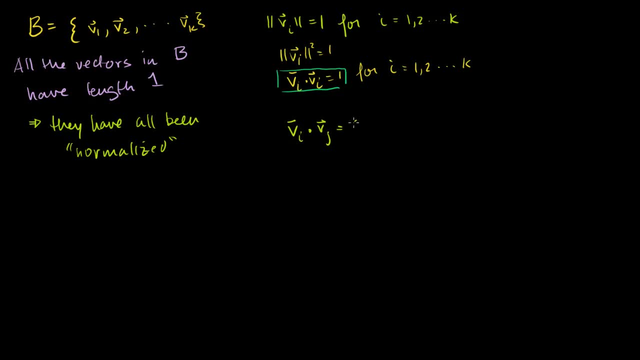 So if you took v2 and dotted it with v1, it's going to be equal to 0.. For i does not equal j, It's going to be 0.. All of these guys are orthogonal. Let me write that down. 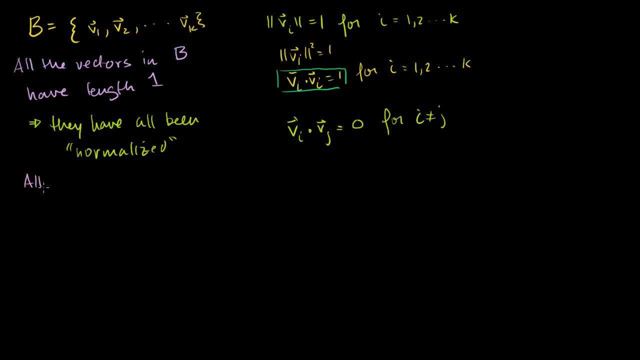 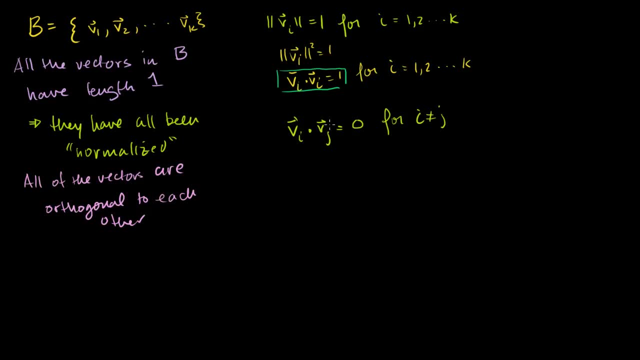 So if you take the dot product with itself, you get 1.. If you take a dot product with some other guy in your set, you're going to get 0.. Or maybe I can write it this way: vi dot, vj for all the members of the set. 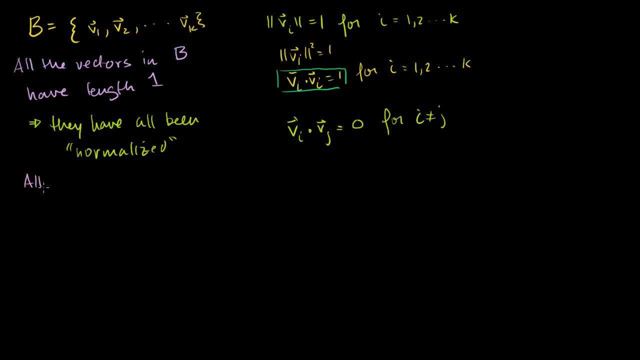 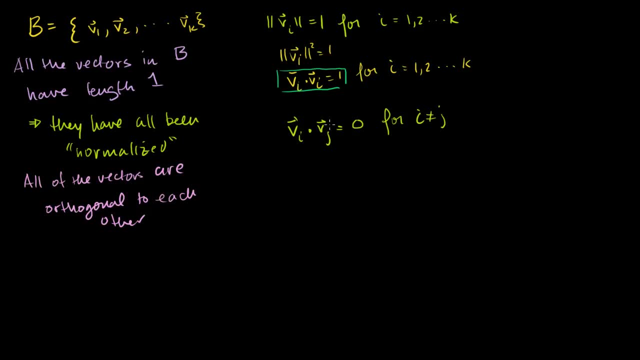 So if you take the dot product with itself, you get 1.. If you take a dot product with some other guy in your set, you're going to get 0.. Or maybe I can write it this way: vi dot, vj for all the members of the set. 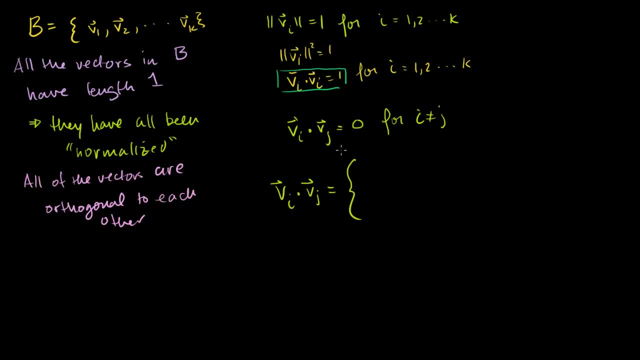 It is going to be equal to. it equals 0 for i does not equal j. And then, if these guys are the same vector, I'm dotting with myself- I'm going to have length 1.. So it would equal length 1 for i is equal to j. 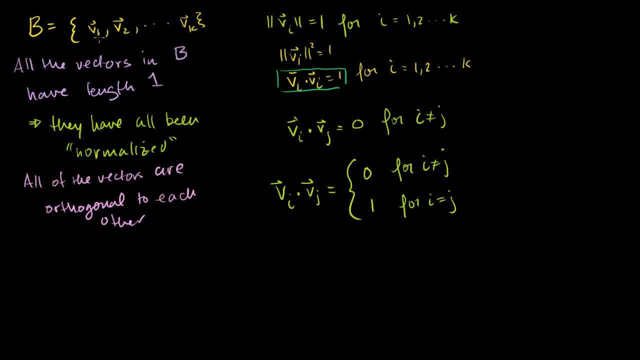 So I've got a special set. All of these guys have length 1. And they are all orthogonal with each other. They're normalized and they're all orthogonal And we have a special word for this: This is called an orthonormal. 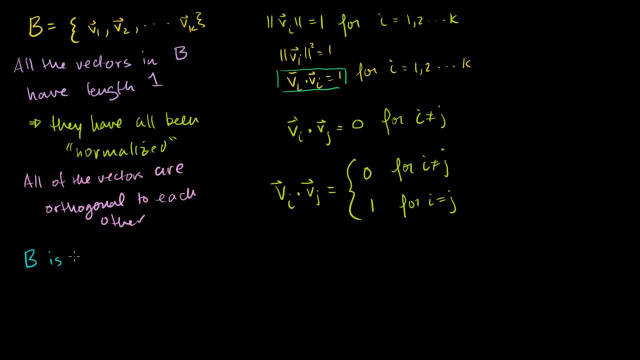 Orthonormal set. So b is an ortho, ortho for orthogonal orthonormal set, Normal for normalized. Everything is orthogonal, They're all orthogonal relative to each other And everything has been normalized. Everything has length 1.. 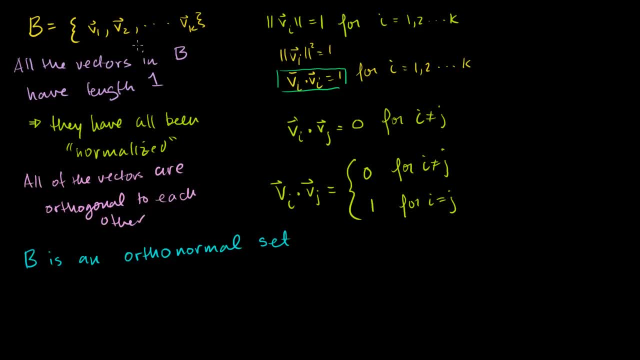 Now the first interesting thing about an orthonormal set is that it's also going to be a linearly independent set, So b. so if b is orthonormal, b is also going to be linearly independent. And how can I show that to you? 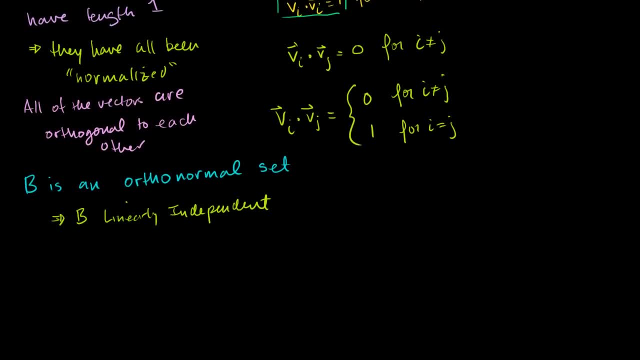 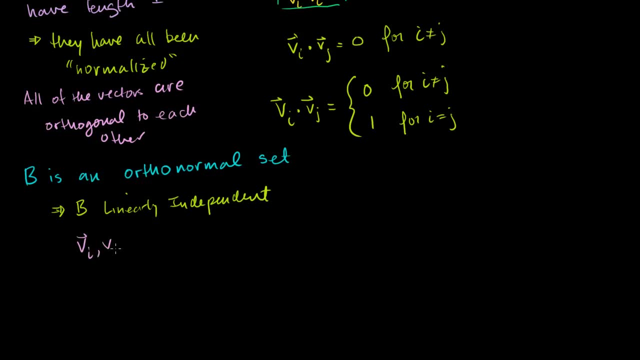 Well, let's assume that it isn't linearly independent. So they're clearly all of you know. let me take vi and let me take vj- that are members of my set, And let's assume that i does not equal j. 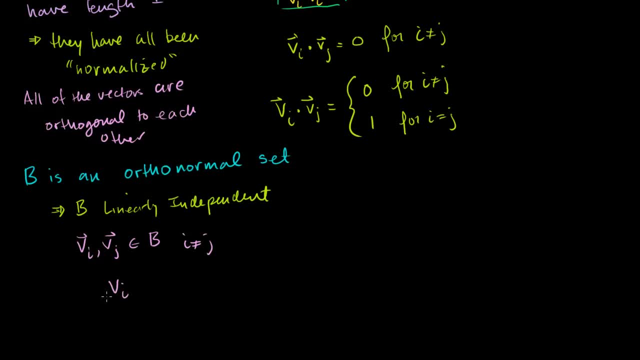 Now we already know that it's an orthonormal set. So vi dot vj is going to be equal to 0.. They're orthogonal. These are two vectors in my set. Now let's assume that they are linearly dependent. 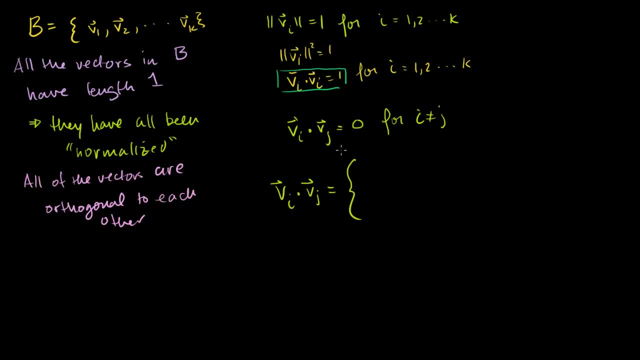 It is going to be equal to. it equals 0 for i does not equal j. And then, if these guys are the same vector, I'm dotting with myself- I'm going to have length 1.. So it would equal length 1 for i is equal to j. 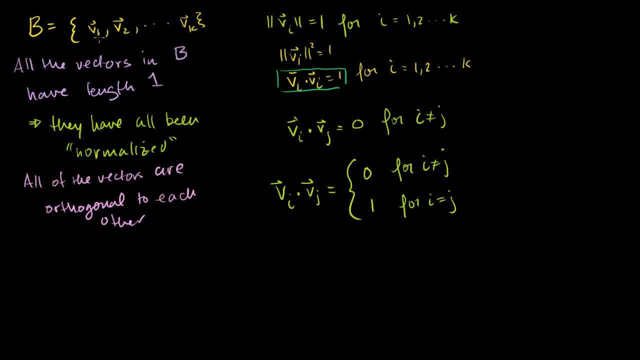 So I've got a special set. All of these guys have length 1. And they are all orthogonal with each other. They're normalized and they're all orthogonal, And we have a special word for this. This is called an orthonormal vector. 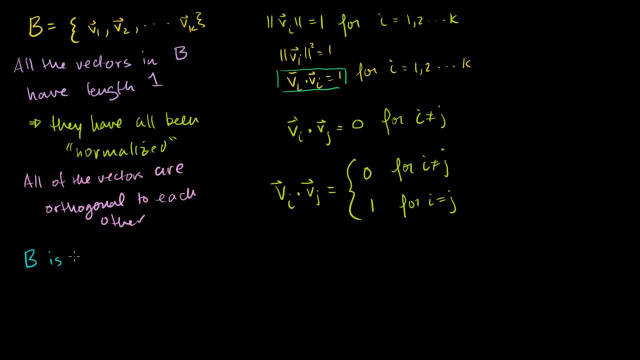 Orthonormal set. So b is an ortho, ortho for orthogonal orthonormal set, Normal for normalized. Everything is orthogonal, They're all orthogonal relative to each other And everything has been normalized. Everything has length 1.. 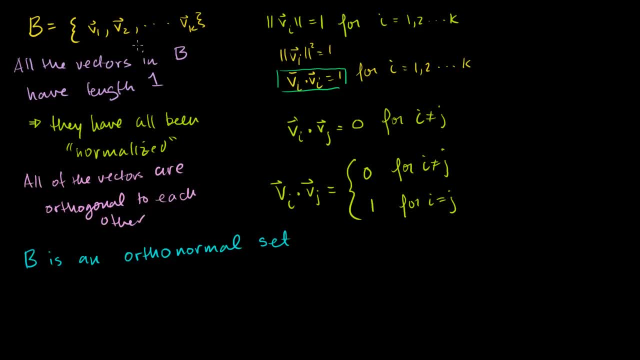 Now the first interesting thing about an orthonormal set is that it's also going to be a linearly independent set, So b. so if b is orthonormal, b is also going to be linearly independent. And how can I show that to you? 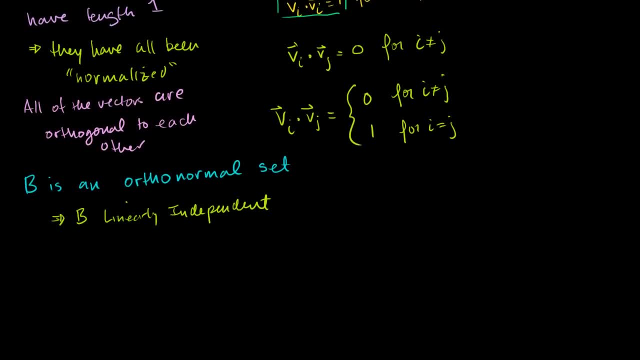 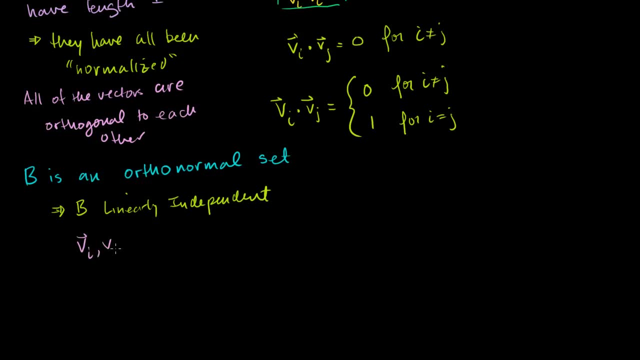 Well, let's assume that it isn't linearly independent. So they're clearly all of you know. let me take vi and let me take vj- that are members of my set, And let's assume that i does not equal j. 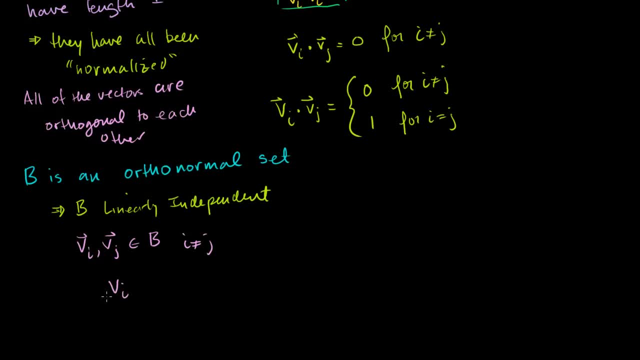 Now we already know that it's an orthonormal set. So vi dot vj is going to be equal to 0.. They're orthogonal. These are two vectors in my set. Now let's assume that they are linearly dependent. 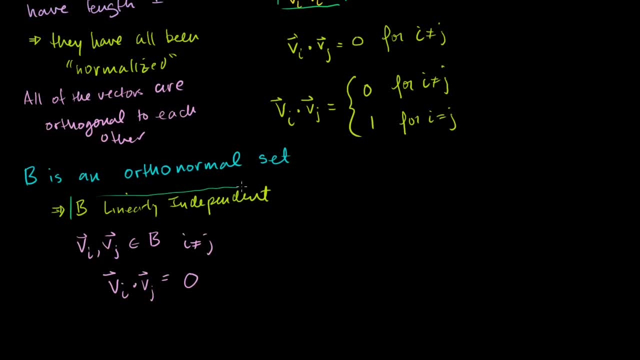 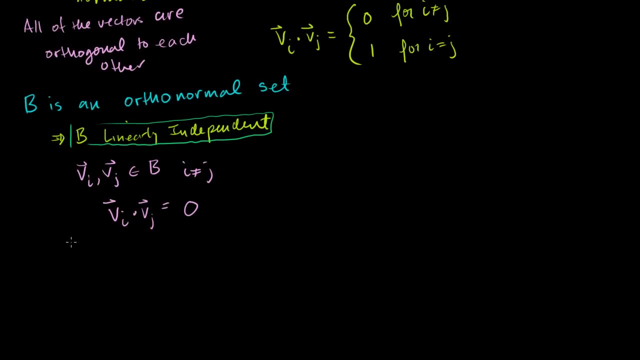 I want to prove that they're linearly independent, And the way I'm going to prove that is by assuming they're linearly dependent and then arriving at a contradiction. So let's assume that vi and vj are linearly dependent. Well then, that means that I can represent one of these guys. 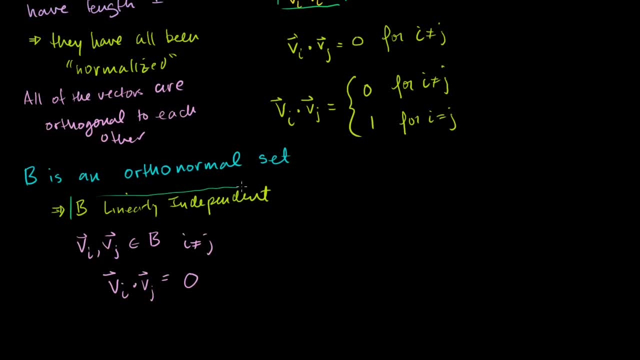 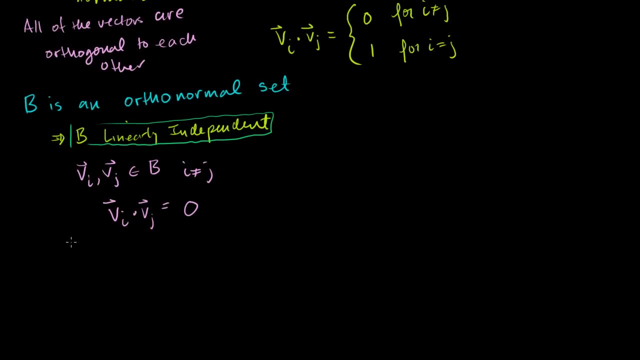 I want to prove that they're linearly independent, And the way I'm going to prove that is by assuming they're linearly dependent and then arriving at a contradiction. So let's assume that vi and vj are linearly dependent. Well then, that means that I can represent one of these guys. 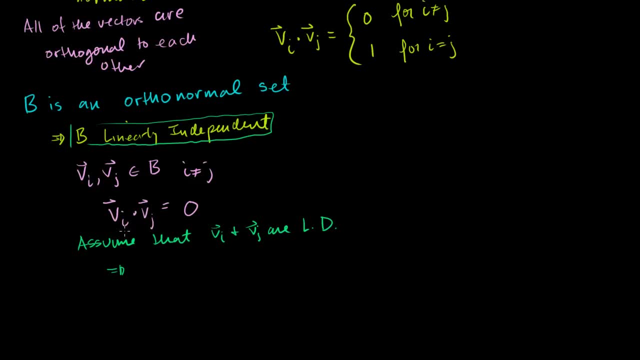 as a scalar multiple of the other, And I can pick either way. So let's just say, for the sake of argument, that I can represent vi. Let's say that vi is equal to some scalar c times vj. That's what linear dependency means: that one of them can be. 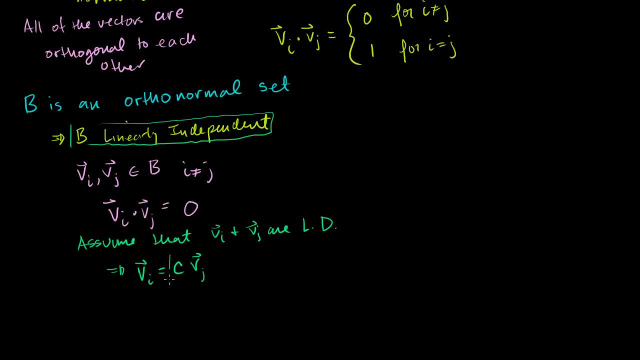 represented as a scalar multiple of the other. Well, if this is true, then I can just substitute this back in for vi, and what do I get? I get c times vj, which is just another way of writing vi, because I assumed linear dependence. 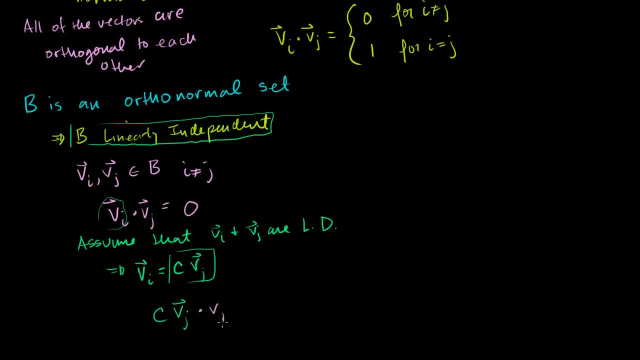 That dot vj has got to be equal to 0.. This guy was vi. This is vj. They're orthogonal to each other. But this right here is just equal to c times vj. dot vj, which is just equal to c times the length of vj squared. 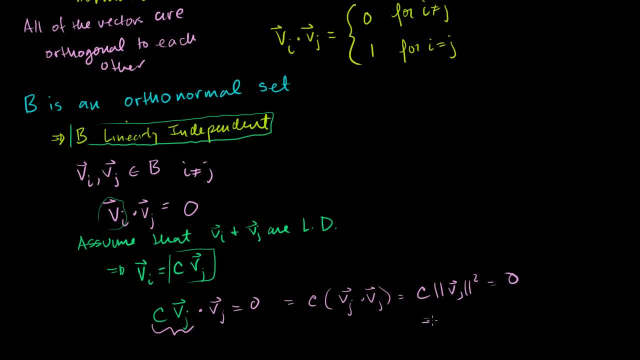 And that has to equal 0.. They're orthogonal, so it has to be equal 0, which implies that the length of vj has to be equal to 0.. If we assume that this is some non-zero multiple and this has to be some non-zero multiple. 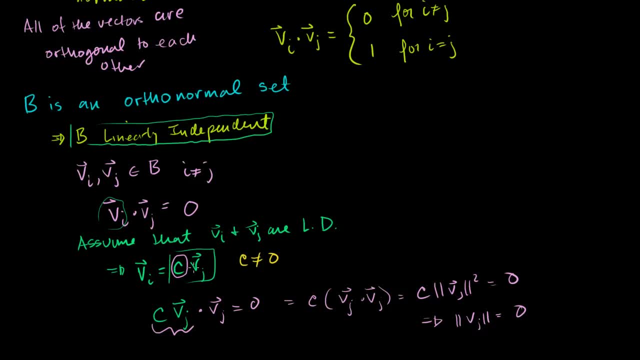 I should have written it there. c does not equal 0.. Why does this have to be a non-zero multiple? Because these were both non-zero vectors. This is a non-zero vector, so this guy can't be 0.. This guy has length 1.. 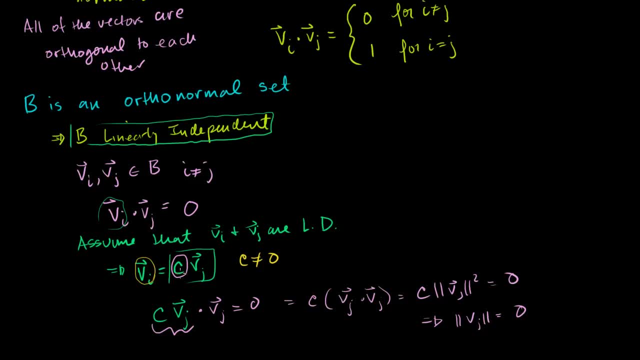 So if this is a non-zero vector, there's no way that I could just put a 0 here, because if I put a 0, then I would get a 0 vector. So c can't be 0.. So if c isn't 0, then this guy right here has to be 0.. 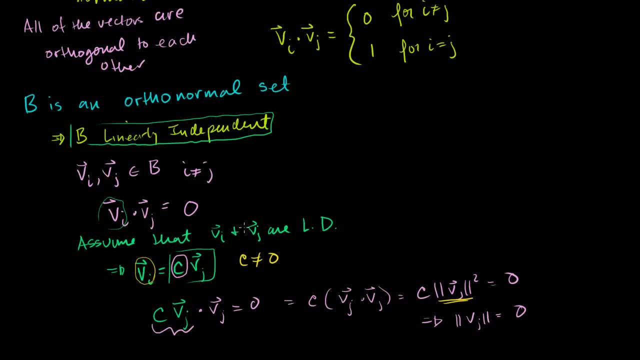 And so we get: the length of vj is 0, which we know is false. The length of vj is 1.. This is an orthonormal set. the length of all of the members of b are 1.. So we reach a contradiction. 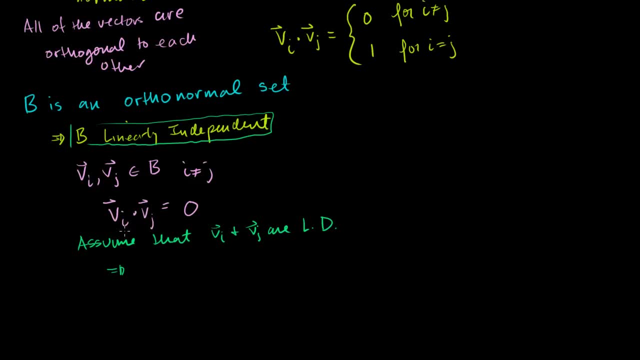 as a scalar multiple of the other, And I can pick either way. So let's just say, for the sake of argument, that I can represent vi. Let's say that vi is equal to some scalar c times vj. That's what linear dependency means: that one of them can be. 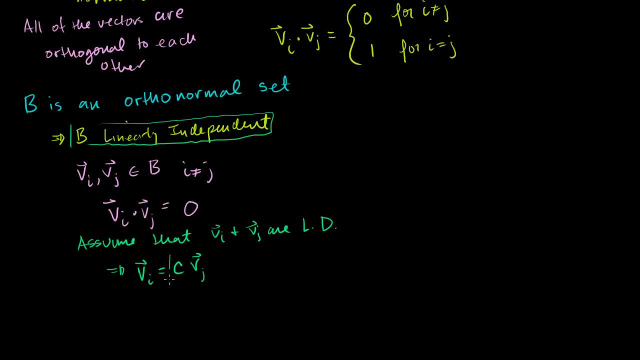 represented as a scalar multiple of the other. Well, if this is true, then I can just substitute this back in for vi, and what do I get? I get c times vj, which is just another way of writing vi, because I assumed linear dependence. 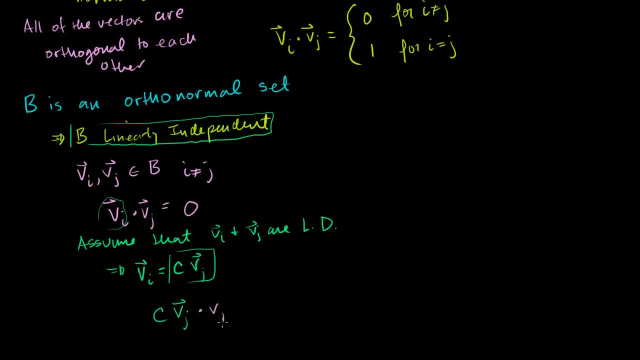 That dot vj has got to be equal to 0.. This guy was vi. This is vj. They're orthogonal to each other. But this right here is just equal to c times vj. dot vj, which is just equal to c times the length of vj squared. 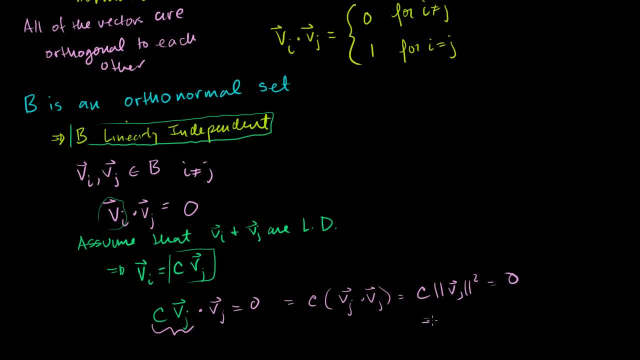 And that has to equal 0.. They're orthogonal, so it has to be equal 0, which implies that the length of vj has to be equal to 0.. If we assume that this is some non-zero multiple and this has to be some non-zero multiple. 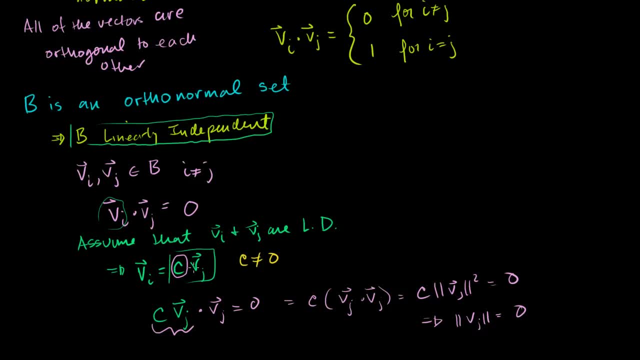 I should have written it there. c does not equal 0.. Why does this have to be a non-zero multiple? Because these were both non-zero vectors. This is a non-zero vector, so this guy can't be 0.. This guy has length 1.. 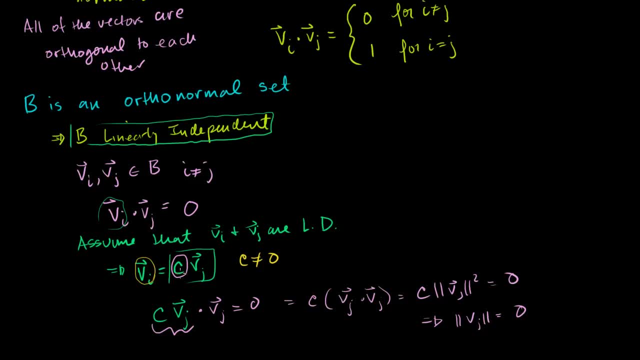 So if this is a non-zero vector, there's no way that I could just put a 0 here, because if I put a 0, then I would get a 0 vector. So c can't be 0.. So if c isn't 0, then this guy right here has to be 0.. 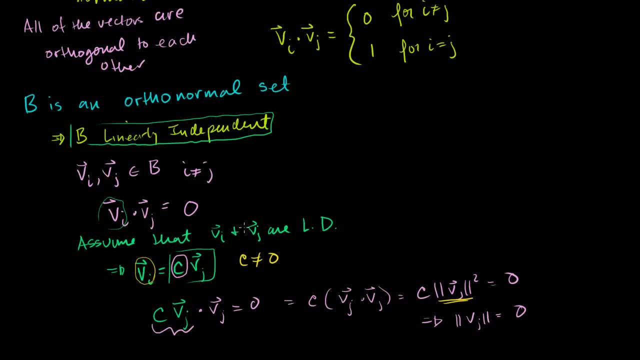 And so we get: the length of vj is 0, which we know is false. The length of vj is 1.. This is an orthonormal set. the length of all of the members of b are 1.. So we reach a contradiction. 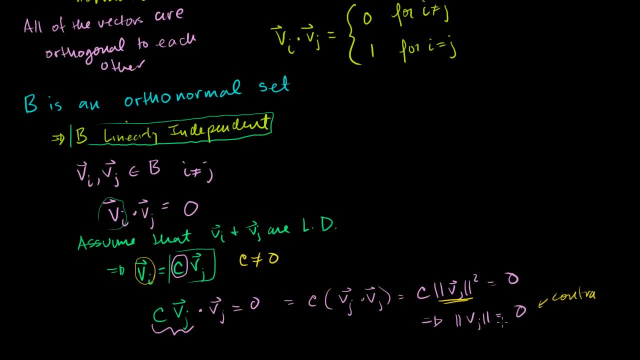 This is our contradiction. vj is not the 0 vector, It has length 1. Contradiction: So if you have a bunch of vectors that are orthogonal and they're non-zero, they have to be linearly independent, which is pretty interesting. 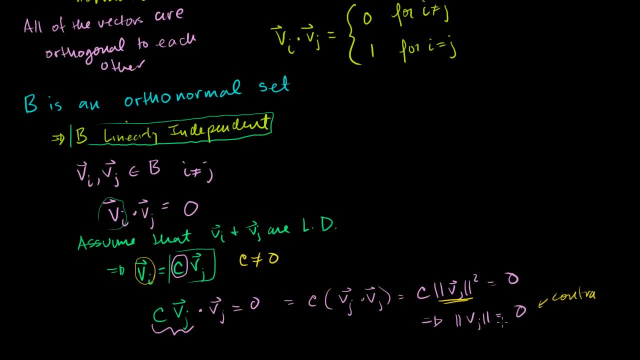 This is our contradiction. vj is not the 0 vector, It has length 1. Contradiction: So if you have a bunch of vectors that are orthogonal and they're non-zero, they have to be linearly independent, which is pretty interesting. 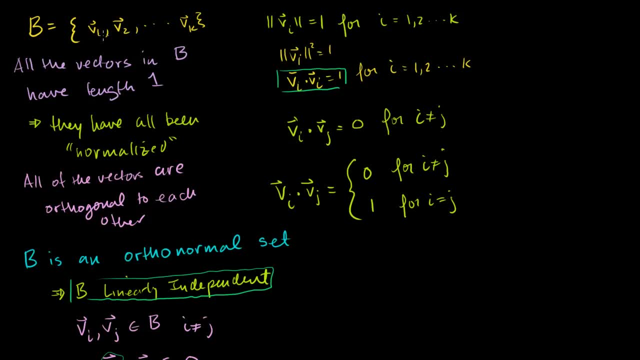 So if I have this set, this orthonormal set, right here, it's also a set of linearly independent vectors, So it can be a basis. It could be a basis for a subspace. So let's say that b is the basis for some subspace, v. 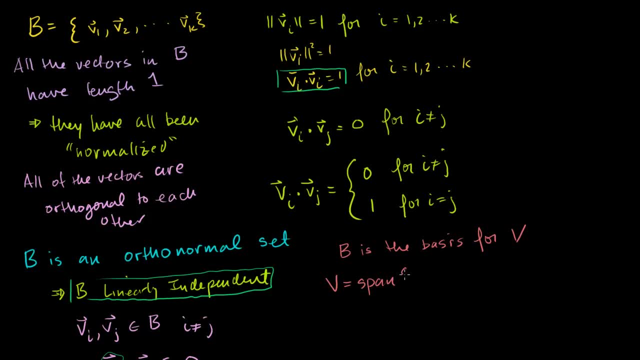 Or we could say that v is equal to the span of v1, v2, all the way to vk. Then we call b. if it was just a set, we call it an orthonormal set. But it can be an orthonormal basis when. 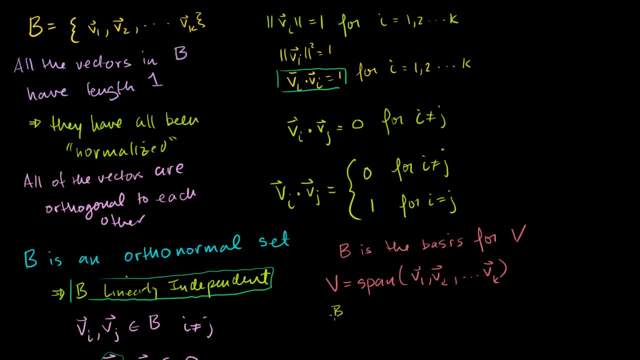 it spans some subspace, So we can say that b is an orthonormal basis for v. Now, everything I've done is very abstract, but let me do some quick examples for you, just so you understand what an orthonormal basis looks like with real numbers. 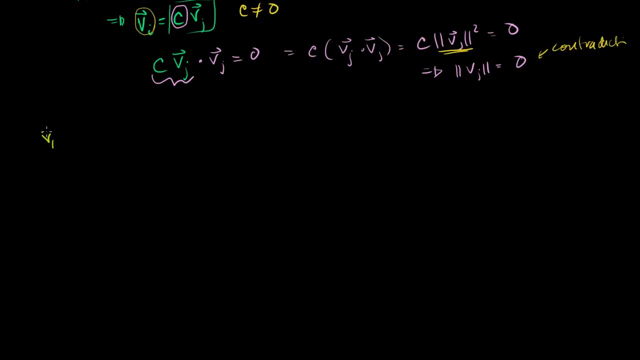 So let's say I have two vectors. Let's say I have the vector v1.. Let's say I have the vector v1. That is, let's say, we're dealing in r3. So it's 1 third, 2 thirds, 2 thirds and 2 thirds. 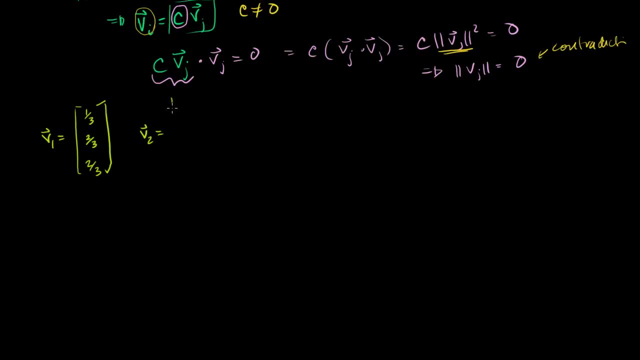 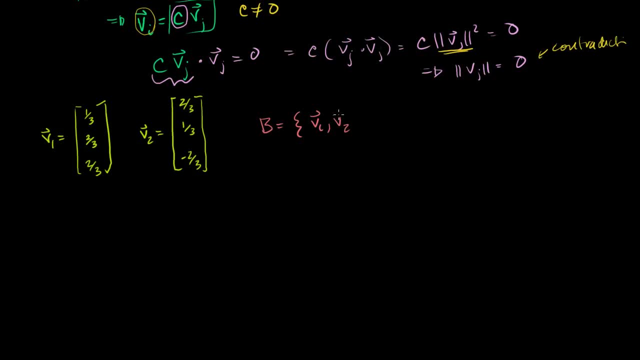 Is the set of v1 and v2.. So the first question is: what are the lengths of these guys? So let's take the length of v1. squared is just v1, dot v1,, which is just 1, third squared, which is just 1 over 9, plus. 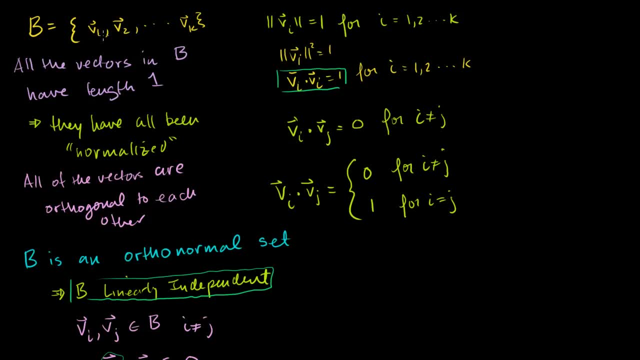 So if I have this set, this orthonormal set, right here, it's also a set of linearly independent vectors, So it can be a basis. It could be a basis for a subspace. So let's say that b is the basis for some subspace, v. 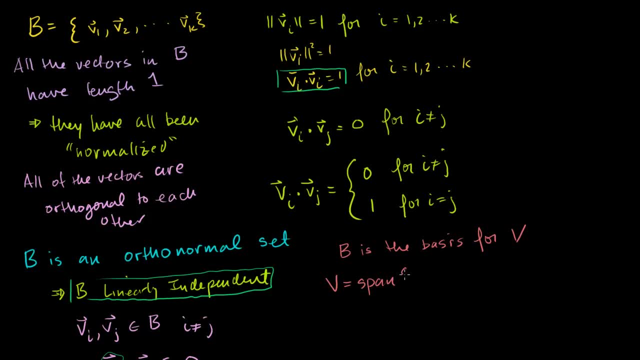 Or we could say that v is equal to the span of v1, v2, all the way to vk. Then we call b. if it was just a set, we call it an orthonormal set. But it can be an orthonormal basis when. 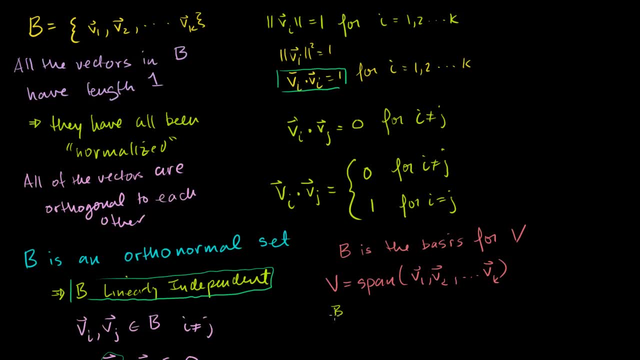 it spans some subspace, So we can say that b is an orthonormal basis for v. Now, everything I've done is very abstract, but let me do some quick examples for you, just so you understand what an orthonormal basis looks like with real numbers. 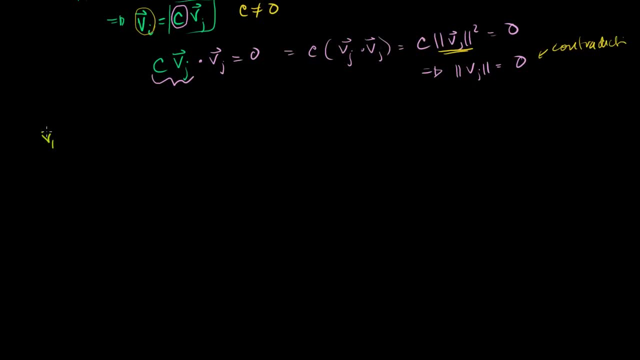 So let's say I have two vectors. Let's say I have the vector v1.. Let's say I have the vector v1.. Let's say we're dealing in r3.. So it's 1 third, 2 thirds, 2 thirds and 2 thirds. 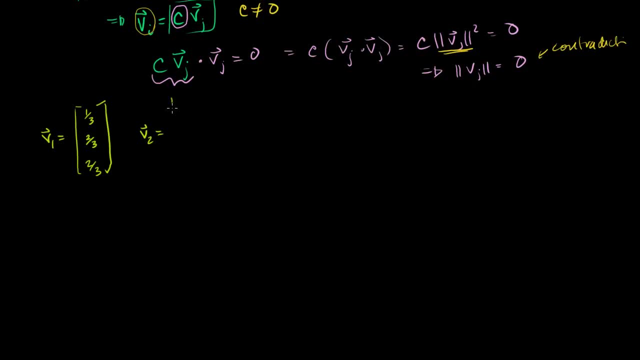 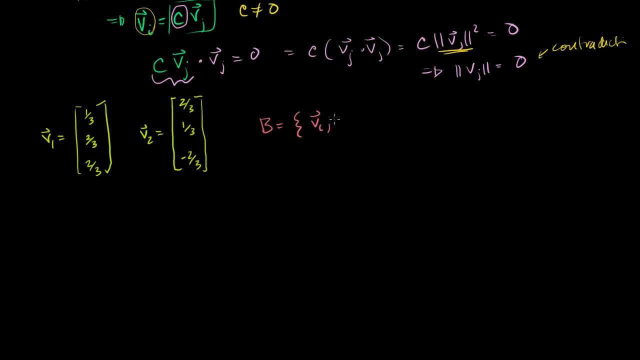 Let's say that b Is the set of v1 and v2.. So the first question is: what are the lengths of these guys? So let's take the length of v1, squared is just v1, dot v1,, which is just 1, third squared, which is just 1 over 9, plus. 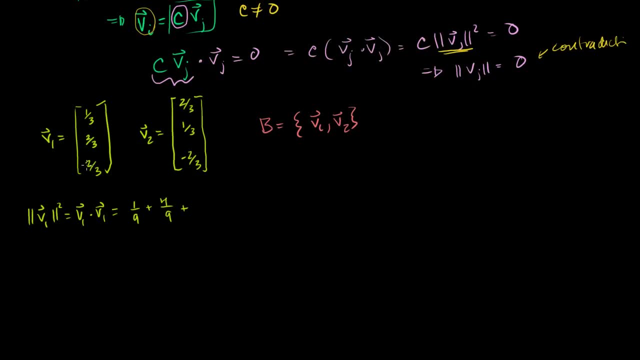 2 thirds squared, which is 4 over 9, plus 2 thirds squared, which is 4 over 9, which is equal to 1.. So the length squared is 1.. Then that tells us that the length of our first vector is: